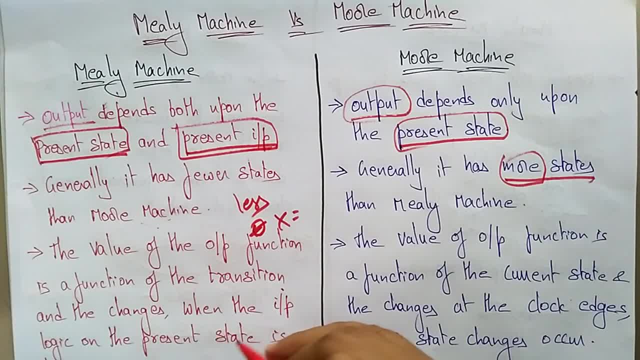 of the transition and the changes when the input logic on the present state is done. So, whereas in the moray machine, the value of the output function is a function of the current state and the changes at the clock edges whenever the state change. 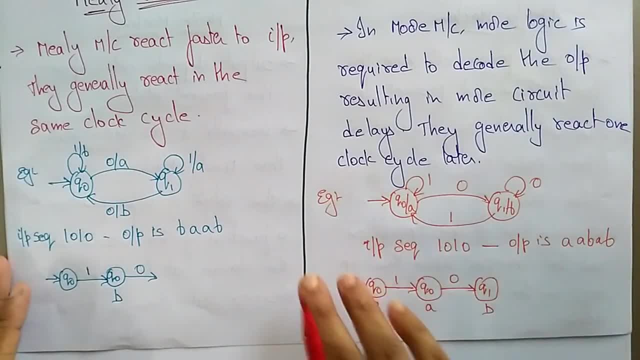 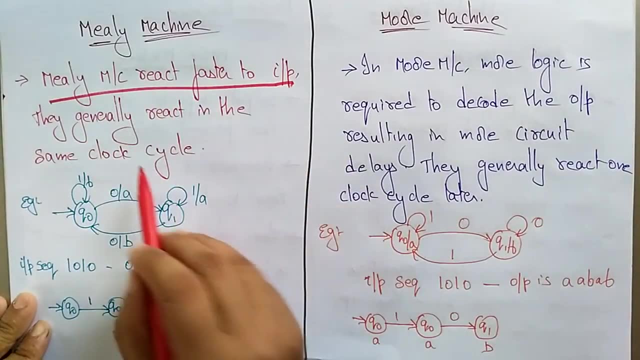 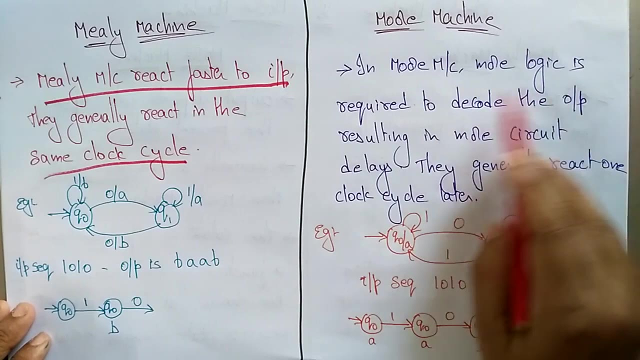 occurs Melee machine. The melee machine is reacts faster to input. Okay, So melee machine reacts faster to input. They generally react in the same clock cycle. Then, whatever the moray machine, In a moray machine, more logic is required to decode the output, which resulting in more circuit delay. 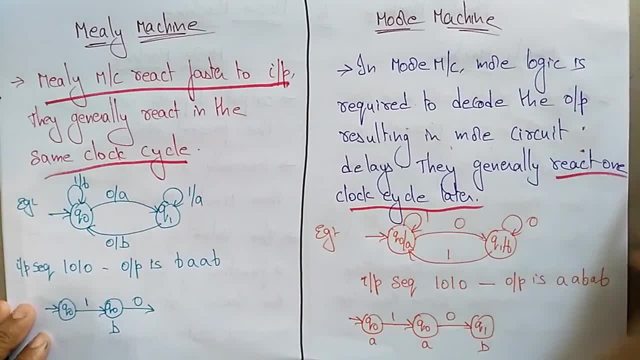 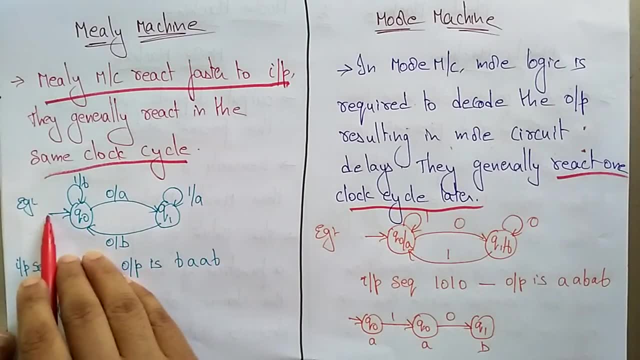 So generally react one clock cycle later. So let us see the example: The melee machine and the moray machine, Simple example. So here I have taken a one state transition diagram. So whatever the input sequence I have taken, the output is different for melee and moray. If I take 1, 0, 1,. 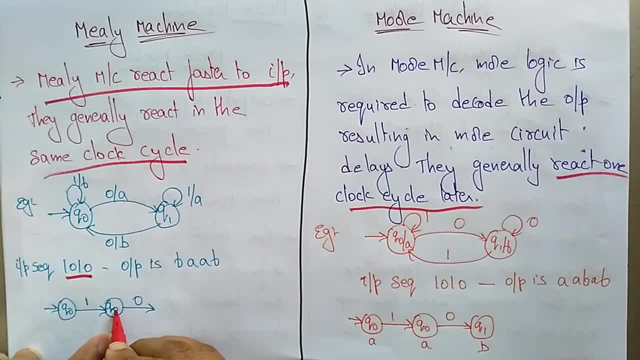 what is the output? So Q naught on 1, it is going to. Q naught only, The output it is generated is B and Q naught on 0.. Going to the state Q 1 and output it is generated is A And Q 1 on 1, this time Q 1 on 1, it is going. 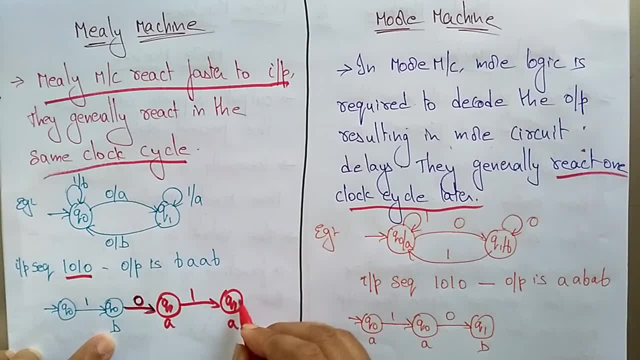 to Q 1 itself and the output it is generated is A And Q 1 on 0, Q 1 on 0, it is going to Q naught and the output it is generated is B, So you got the string as B, A, A, B, Whereas coming to the 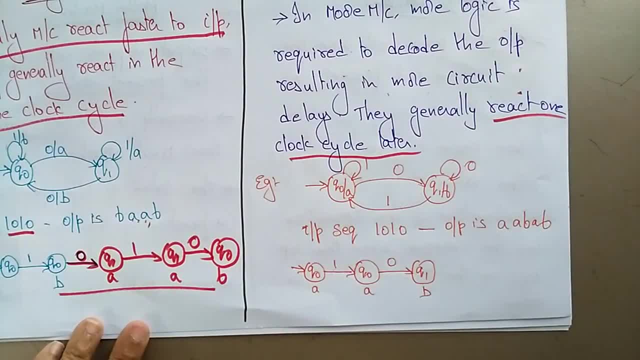 moray machine, So state consisting of state and the output as well, Because it is depends only on the input, the present state It is not, and depends upon the input. It depends upon the present state, only Here the input sequence. they are given 1, 0, 1, and then what is the output? Q naught on 1,. Q naught on 1,. 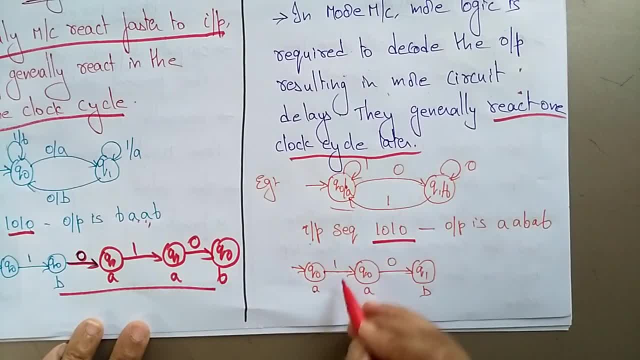 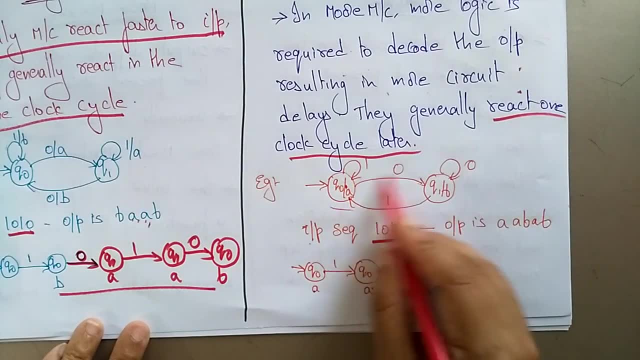 initially it is A because the Q naught output is A Q naught on 1, it is going to Q naught itself. The output of Q naught is A Q naught on 0, it is going to Q 1.. The output of Q: 1,.